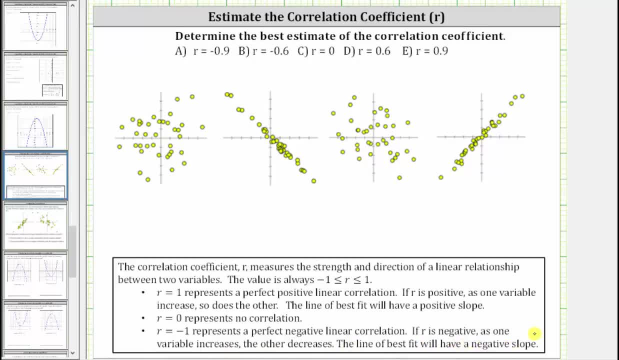 the other decreases, The line of best fit will have a negative slope. Let's begin by sketching a possible line of best fit for each scatterplot. Notice for the second scatterplot and the fourth scatterplot. it's very easy to sketch a line of best fit. 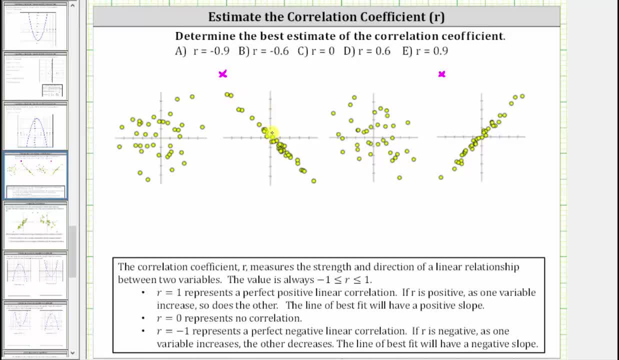 which again is a line that best describes the behavior of the data. Notice how for this scatterplot. if we sketch this line here, it's a very good representation of the data because all the points are very close to the line of best fit. 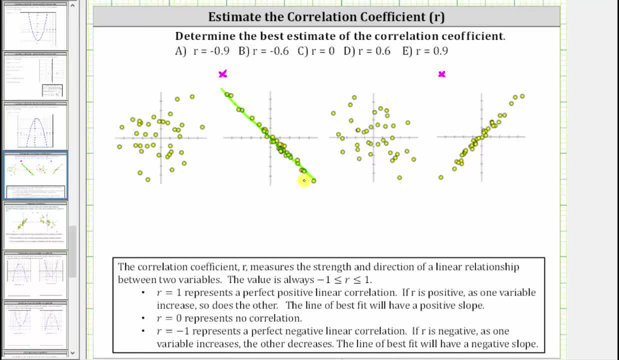 which means we have a strong correlation, And because the line of best fit is a negative slope, or because as one variable increases, the other decreases, we have a very strong negative linear correlation and therefore r is going to be close to negative one. So, looking at the choices, 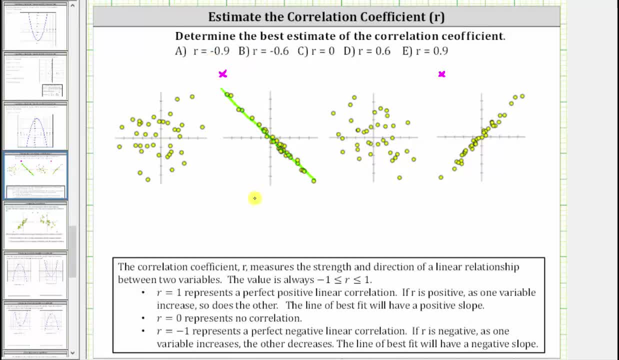 let's select a. r equals negative 0.9.. This is where this line of best fit will get the positive slope. What we do is we're going to look at the correlation between b and r And we're going to look at the number of sides. 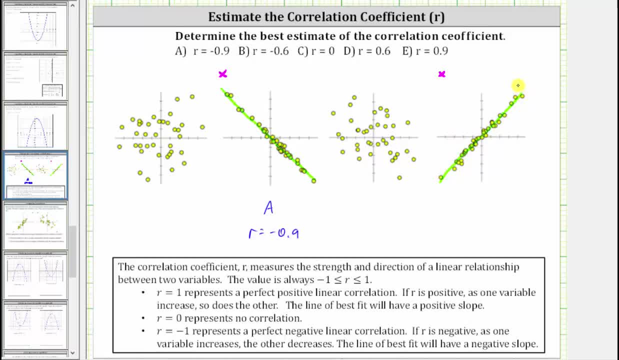 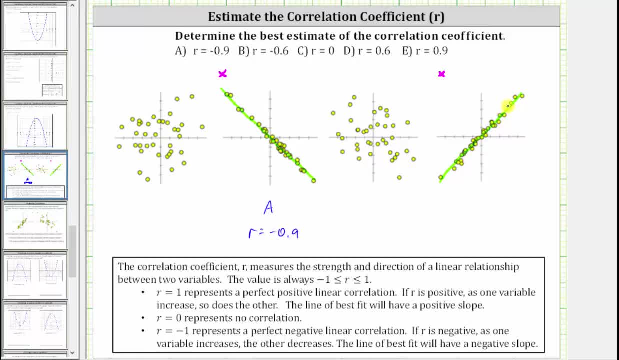 into our positive slope. Now, if we get a line of best fit, it will represent the behavior of the data. It might look something like this And once again notice how all the points are very close to the line let's select: E. r equals positive 0.9.. 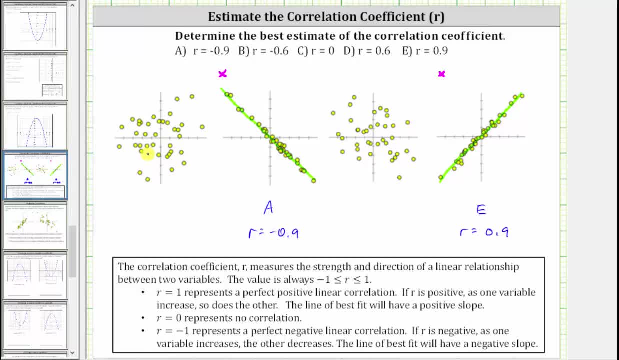 Now let's take a look at the remaining two scatterplots. Notice: for the remaining scatterplots the points are more scattered. So for the first scatterplot, if we were to sketch a line of best fit, it might look something like this: 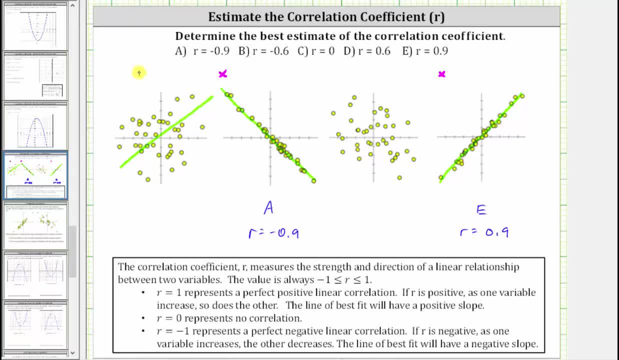 Notice how the slope of this line is positive and therefore r is going to be greater than one or positive. but because the points are not as close to the line of best fit as they were for this line of best fit, r is not going to be as close to positive one. 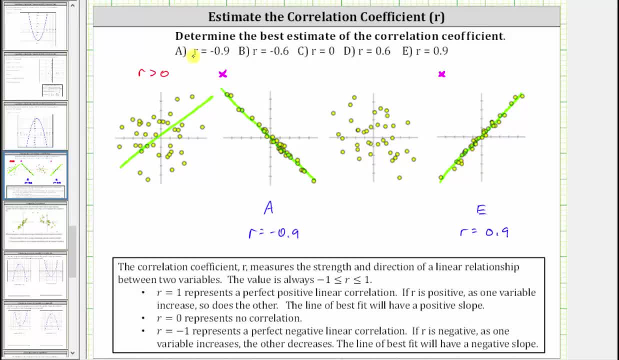 for this scatterplot, as it was for this scatterplot. So, looking at the choices, let's select D. r equals positive 0.6.. We still have a positive linear correlation, but it's not as strong as this scatterplot here.